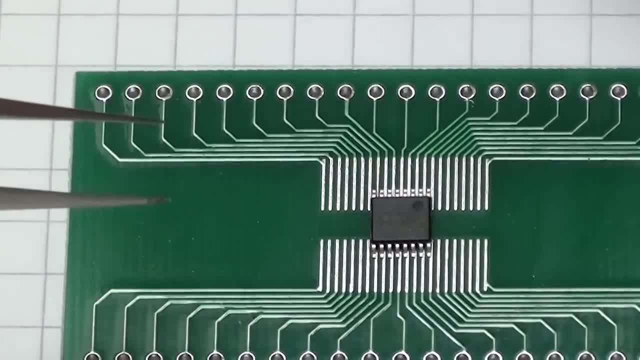 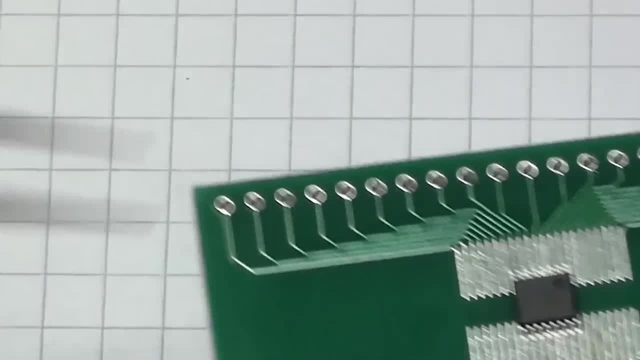 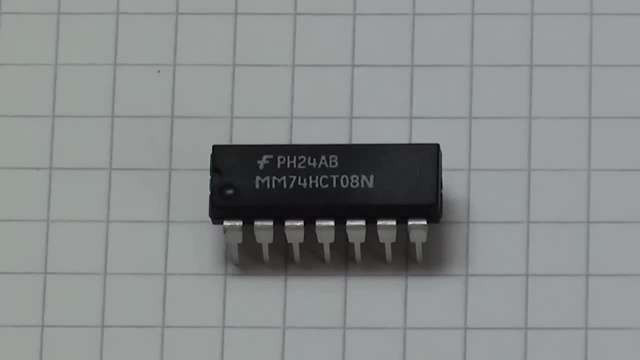 that certain types of chips that we need to use are only available in SOIC form and that means in that packaging format, which means that we would have to use a converter board like this. So we're going to use the DIP packaging format for our experiments, So each chip has 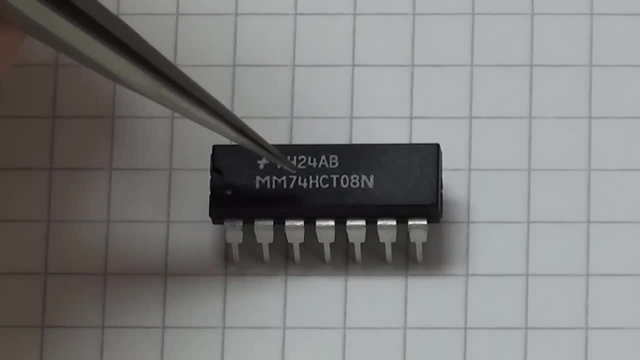 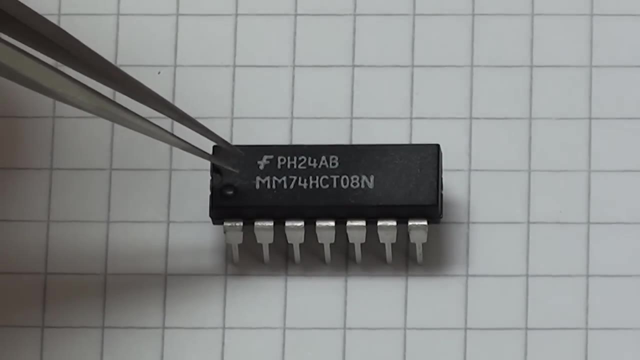 an identifying number, and here we can see that this one is the MM74HCT08N. The letters all mean something. The MM in this case refers to the manufacturer, which is Fairchild Semiconductor. It could also be letters like SN, which would refer to Texas Instruments, for example The 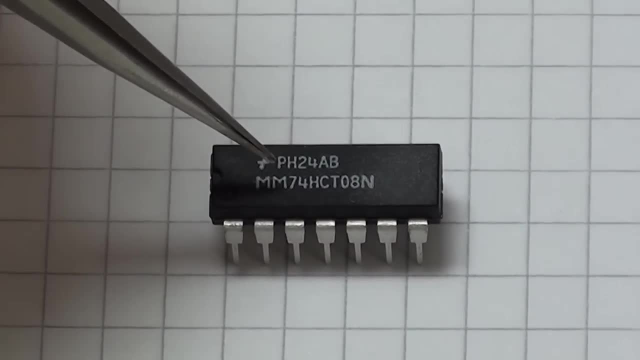 74 is the way that you know. I suppose this is the giveaway in terms of finding the number that makes sense on your chip. The 74, and we skip the letters in between- 7408 refers to the particular type of chip. This is a quad 2 input and gateway chip. 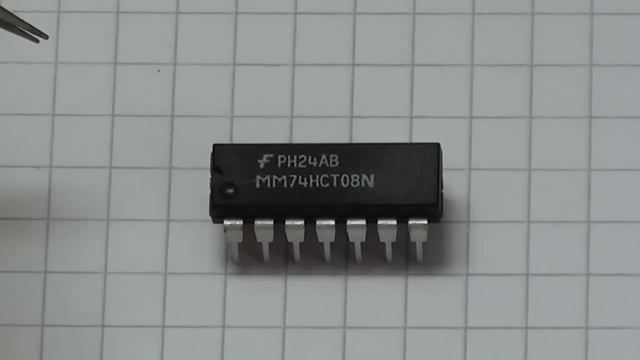 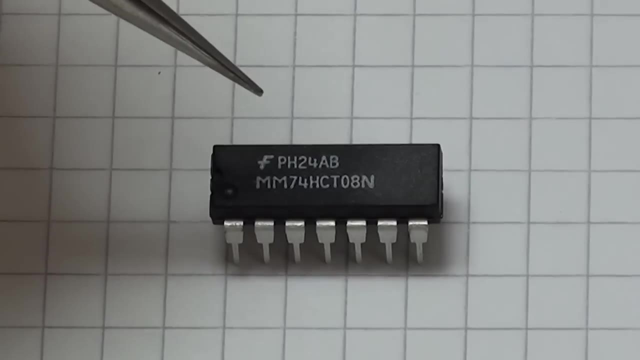 So there's four 2 input and gates in this particular chip. The N at the end refers to the packaging type. So we know that this is a DIP packaging type. So the N refers to DIP, the dual inline packaging type. And finally we have the HCT in the middle, which refers 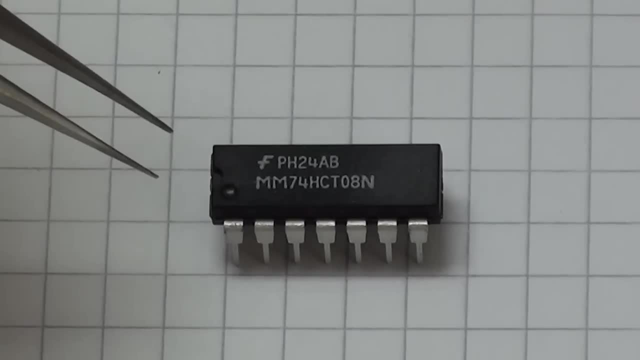 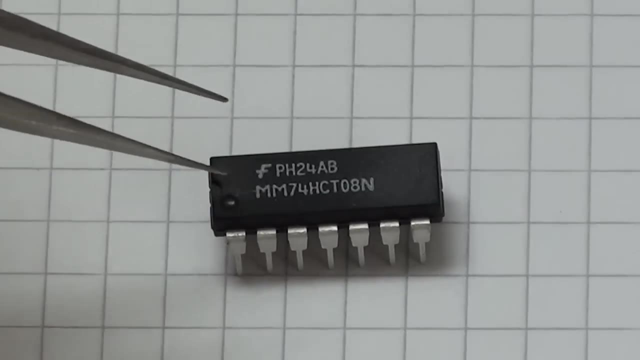 to the particular logic family that the chip belongs to. In this particular case, it's a high speed CMOS with TTL logic levels. So this is the particular logic family that the chip belongs to. So this is the particular type of chip that we're going to be using. 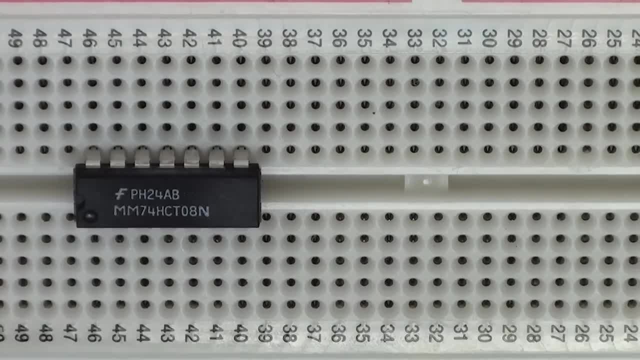 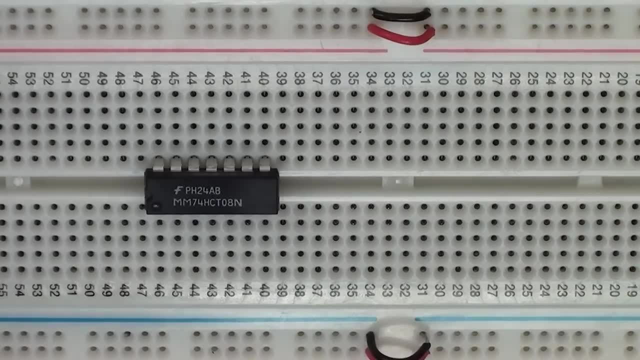 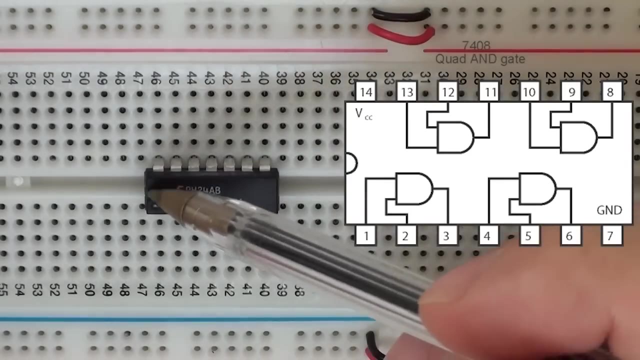 for our experiments. First thing we need to do is we need to connect up the power to the chip. So I've set up the rails so that we have easy access- And this particular chip, pin 7, has to be connected to ground and pin 14 has to be connected to VCC. So here we're going to connect pin 14. 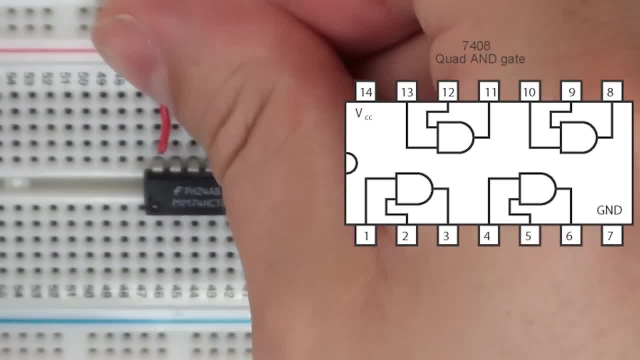 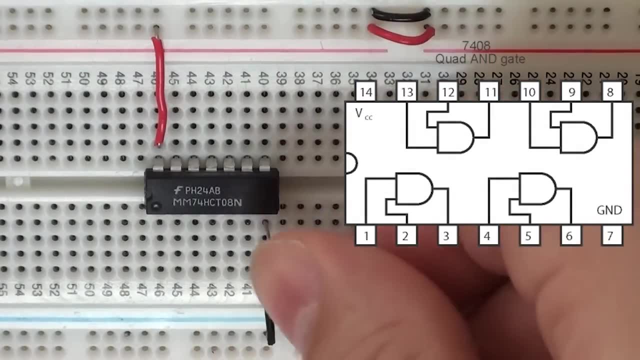 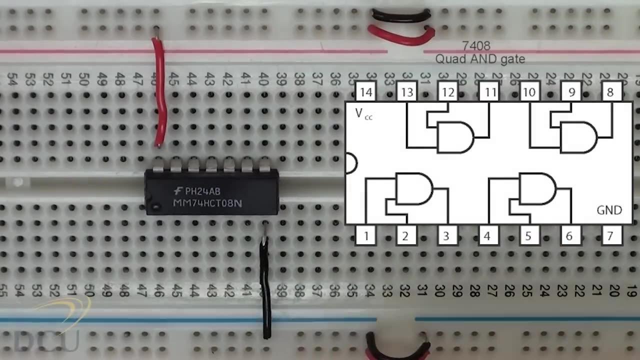 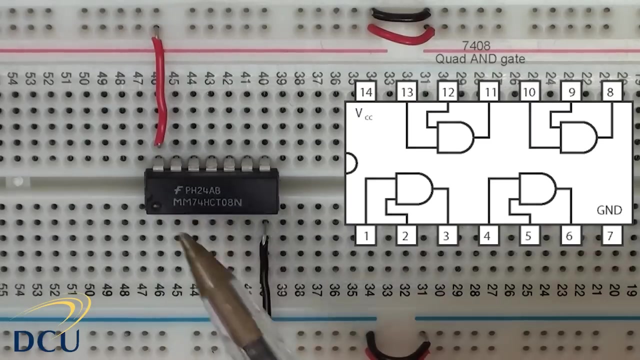 to VCC and pin 7 to ground. So our chip is powered. I haven't connected the supply yet, but the chip is powered. And then we have. now we have our input on pins 1,, 2, and 3. again, We can tell our first pin. 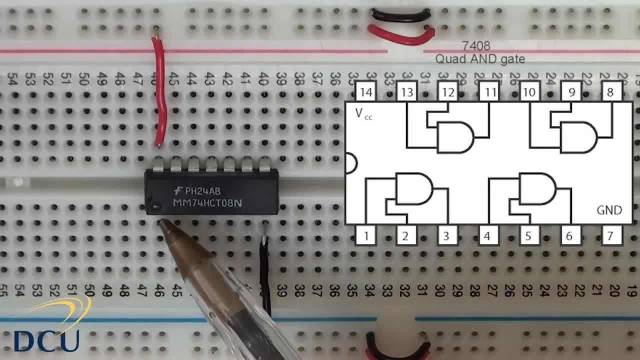 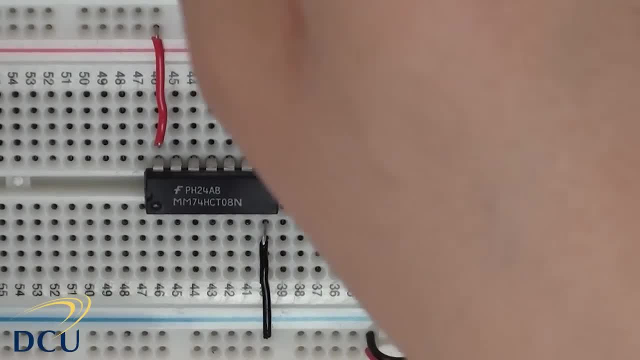 by the circle that's just visible there on the top of the chip. We have pin 1, 2 are inputs and pin 3 is our output. So we need some way of seeing our output. So we're going to use an LED for this. 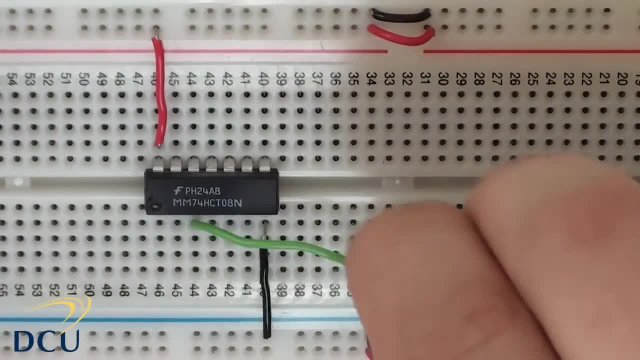 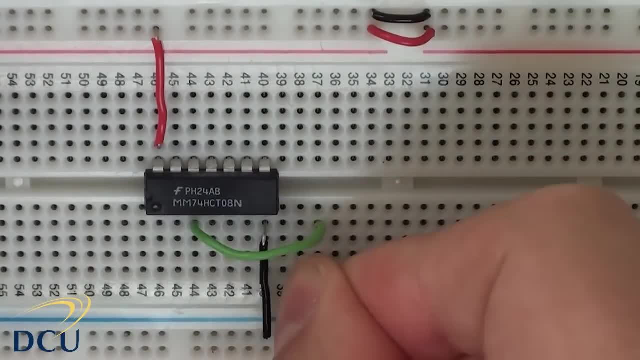 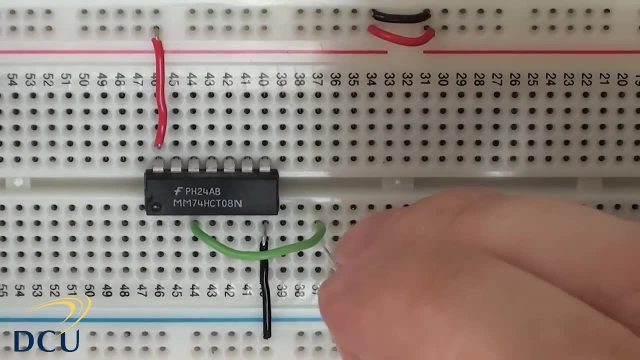 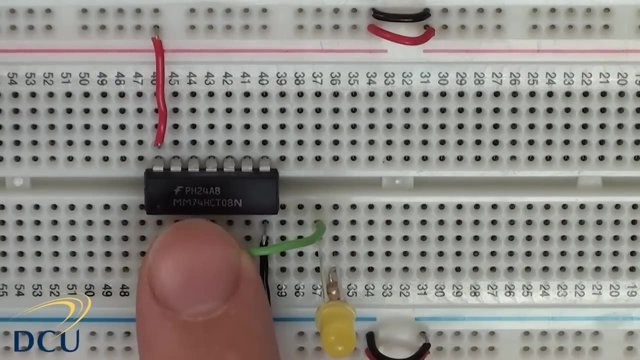 And I'll just use a small resistor tied to ground, as before, And then we just bridge that Again, remembering the longer leg is the positive is connected to pin 3. And the shorter leg is connected through ground, sorry to ground through the little resistor. 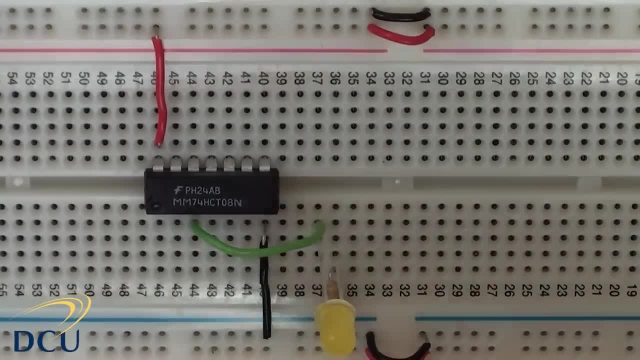 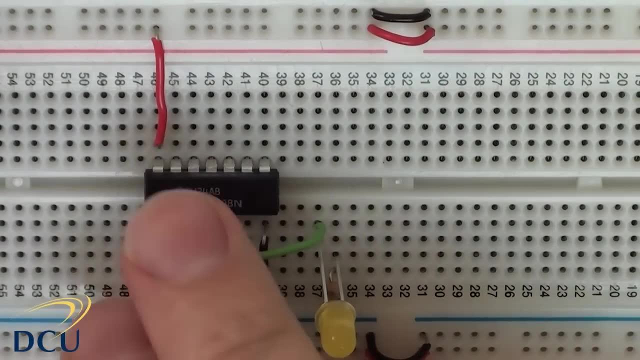 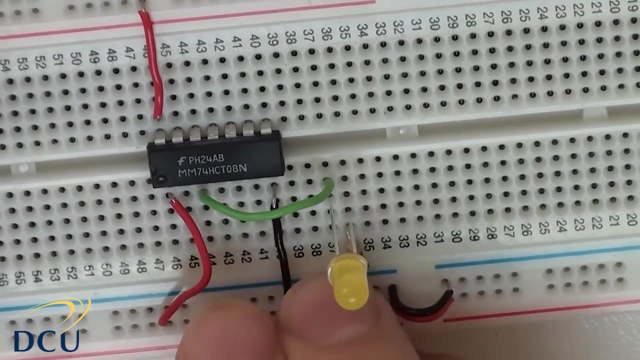 So now we have our circuit and we can test it And we can say: well, let's connect both of our inputs to be high And in this particular case, when we turn on the power, you should see very quickly that we get a value of our 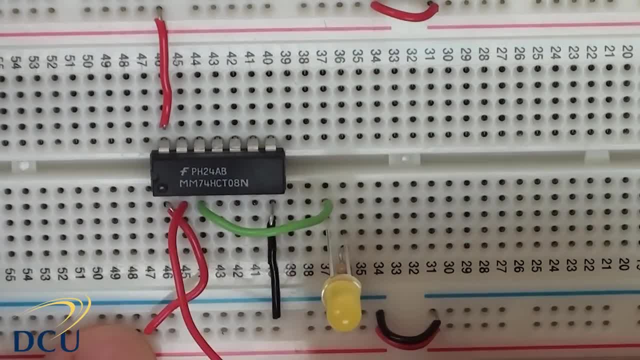 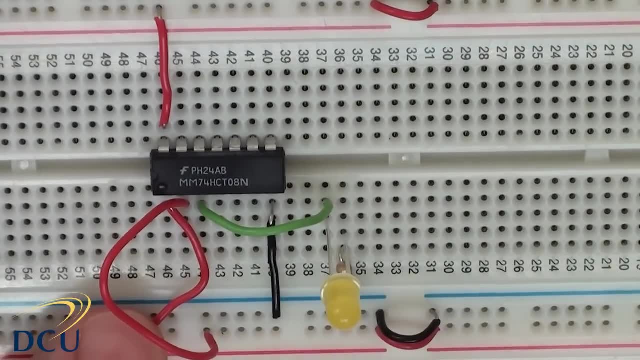 LED should light. So if it pins 1 and 2, both connect to VCC to 5 volts, And when we turn on our power supply now, you'll see that the LED lights. I'm just going to leave the power supply. 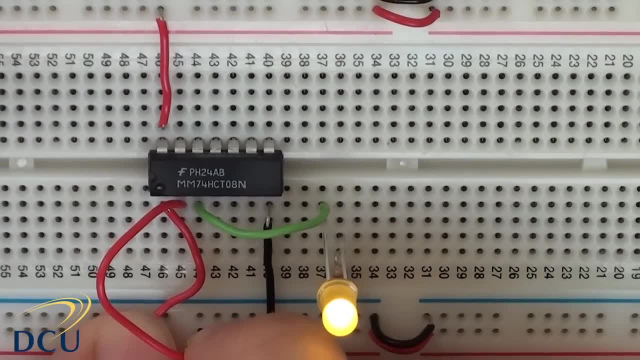 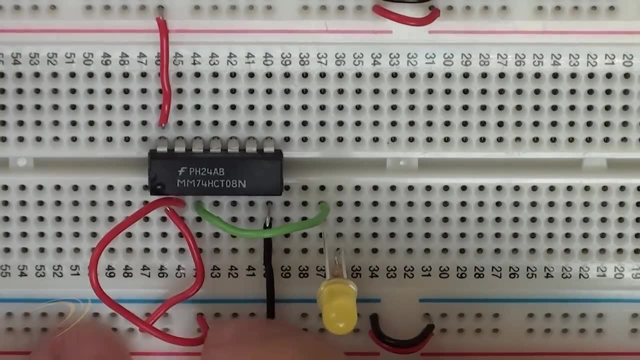 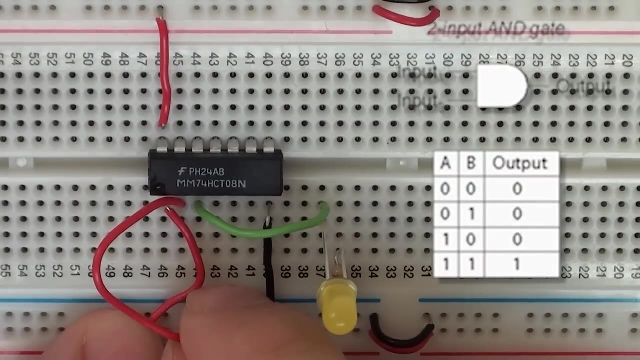 lit and I'm going to disconnect one of my inputs and connect it to ground, And there you'll see that now that it's connected to ground, the LED is off. If I do it on the same with the other pins, it'll have the same effect. You'll know from the true table for an AND gate that both inputs have. 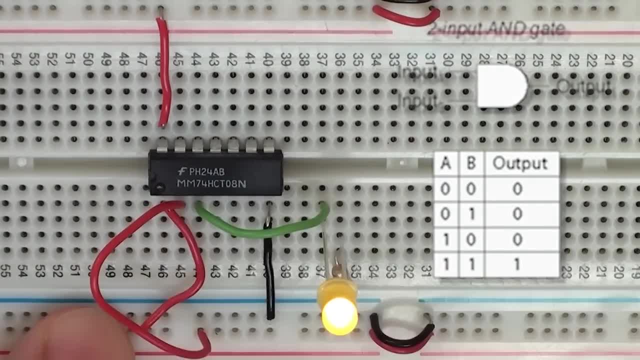 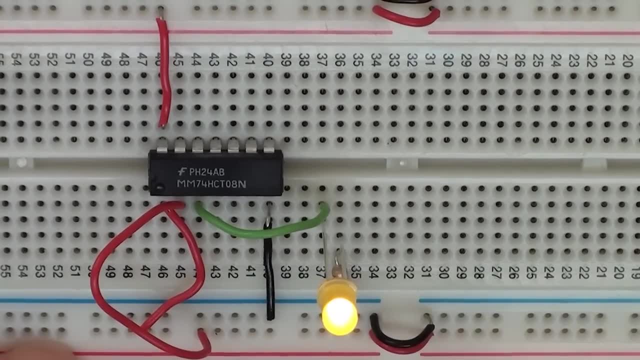 to be high for the LED to be lit. So if I again set both inputs to be high, then we can light our LED like this. Now what we're going to do is we're going to say, well, moving these wires around is a little bit awkward, So let's connect in two switches. I'm just going to turn off the power. 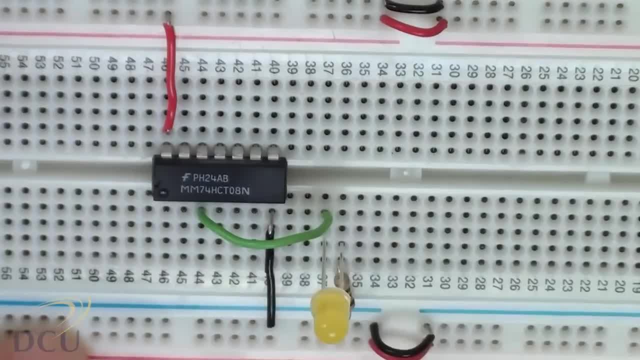 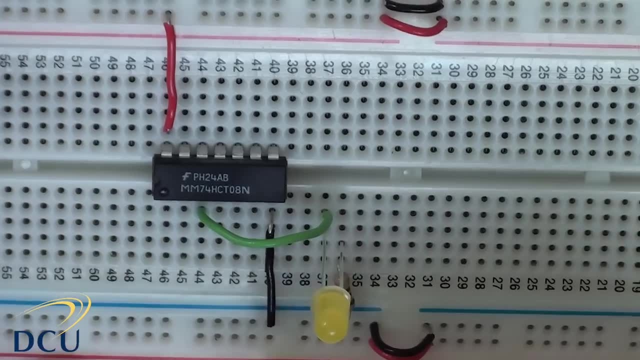 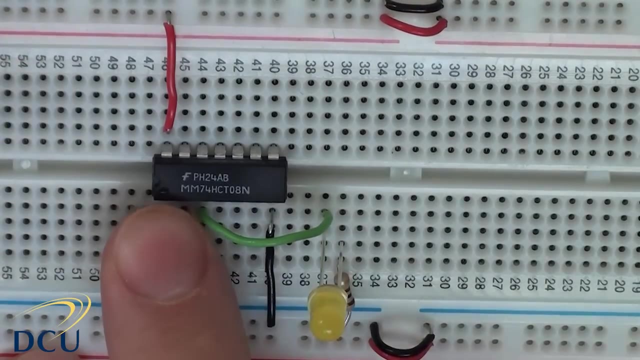 and connecting two switches. I'm going to use these push button switches and just make sure you have them in the correct orientation And we're going to connect these across to connect the first one so that it's touching pin. it's in the same row as pin 1.. So that means 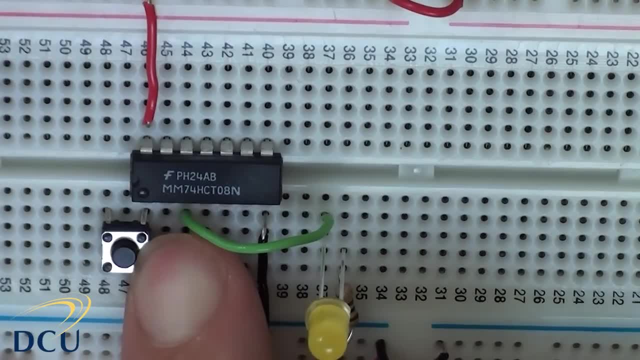 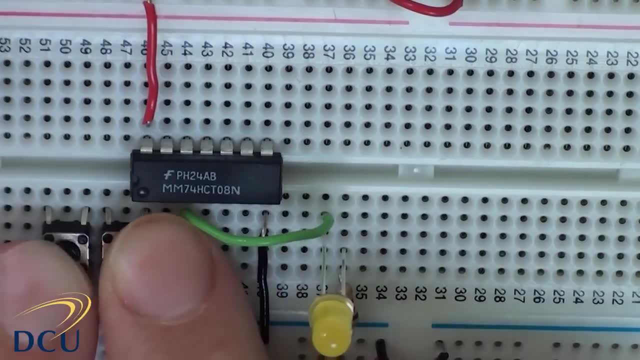 that I'm only going to have to connect to the other side of the of the switch. Just make sure that they're a little fiddly. they might come out, And I'm going to put the other switch right beside it. Okay, so we have two switches. Push them in well into the boards And these buttons are going. 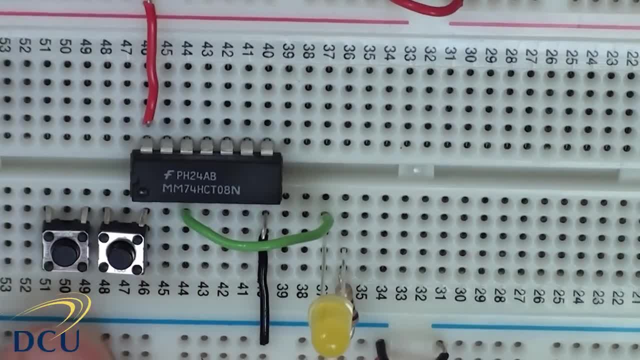 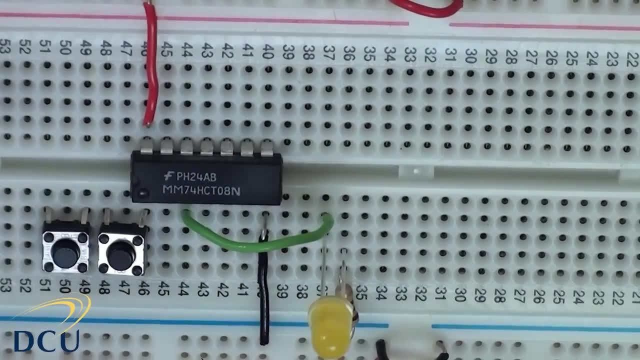 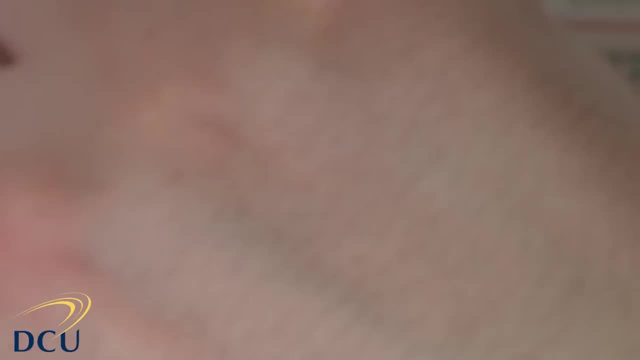 to provide my inputs. And we should see that when our circuit is connected, that we get a high only the LED lights. we get a high only when both buttons are pressed at the same time together. So we need to connect up to say well, well, let's say well, let's connect up a high to this. 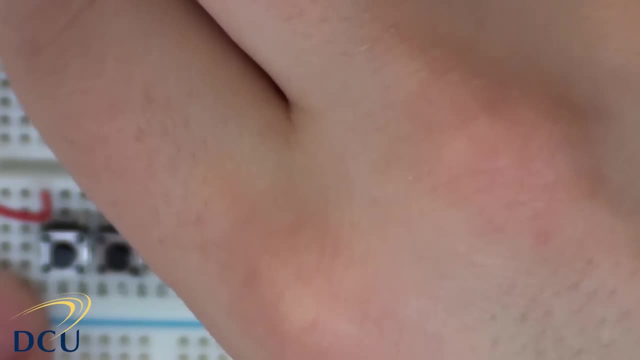 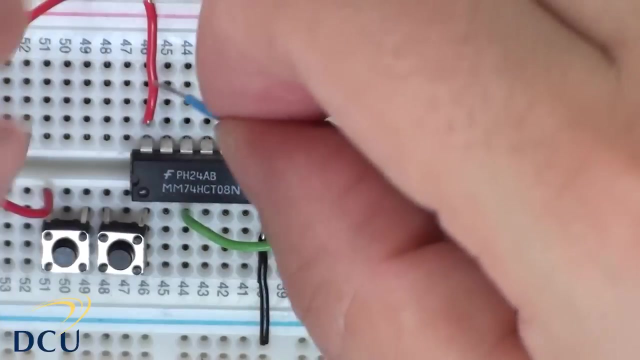 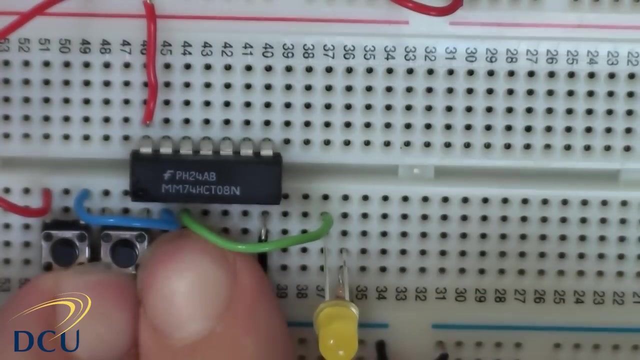 to this side of this pin. we should go into the right place And to the other side let's connect up our goes in to the other side of our switch. Let's connect that to the second input And the second switch is already connected into pin one. 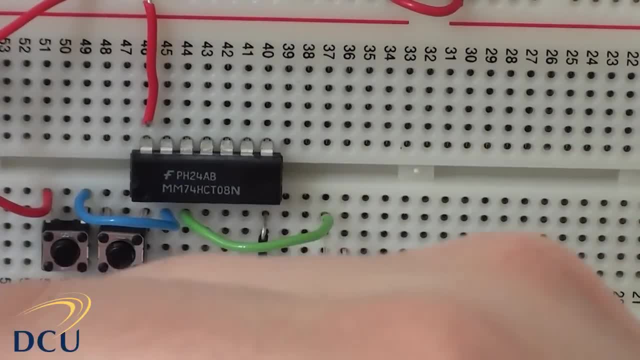 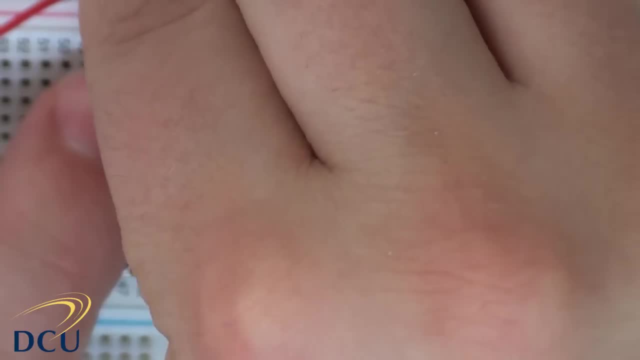 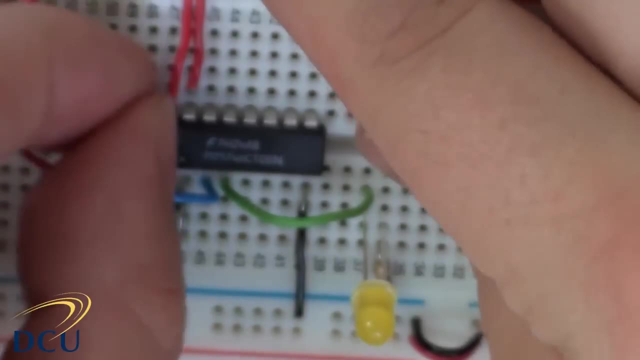 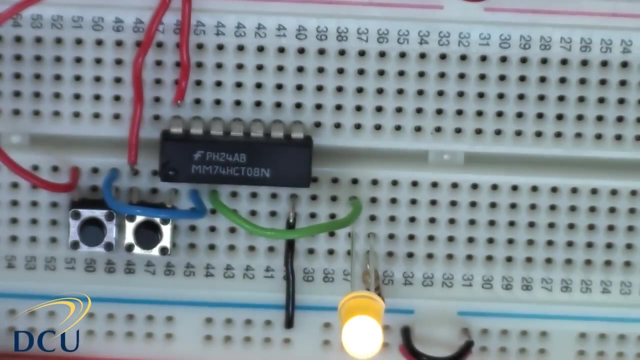 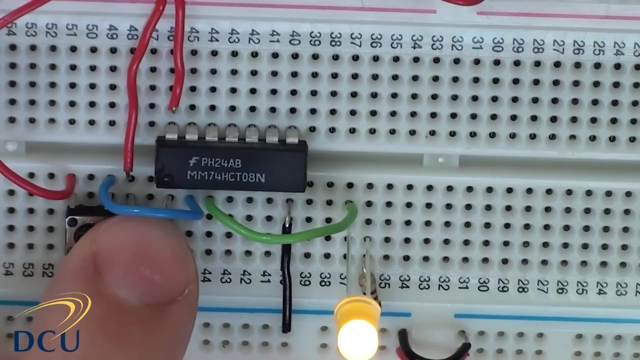 And we just need to connect the other side of it into our higher Okay, Okay, reaches to up to reach. Now we turn on our circuit, you're going to see something unusual happen. It doesn't work. And if we press the buttons and we will see that, well, the LED nearly always stays on. So it's.